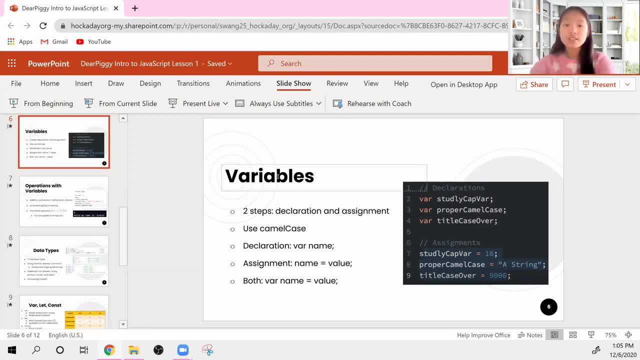 this first video, we're going to be working with just var. So for variables, there are two steps. There's the declaration and the assignment. We can do this in two separate lines, or we can do it in one line. Either way, it doesn't matter. Now, variables are really really useful, guys, because 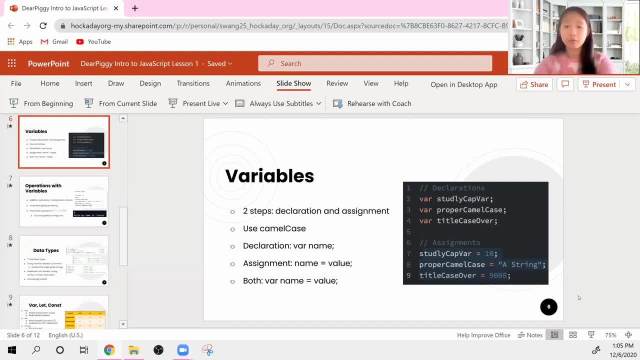 they can store values and can be reused over and over again. So say, I want to have a certain number of puppies. you could say, but I don't want to have a certain number of puppies, So I'm going to write that number over and over and over when I want to reuse it in my code By assigning the. 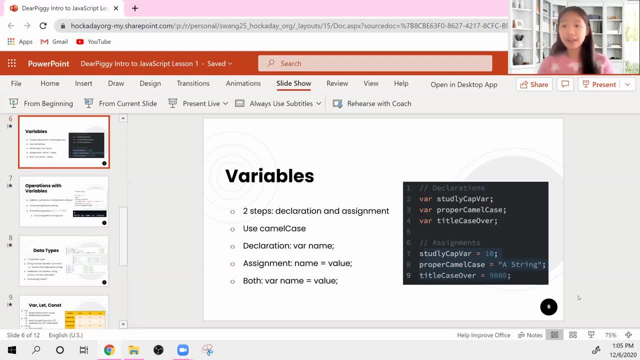 value to a variable. we can use the value, we can use the variable over and over, and that would make our lives so much easier. Last thing that we want to know about before we go ahead and get started is camel case. Every single coding language has its own coding standard. There's 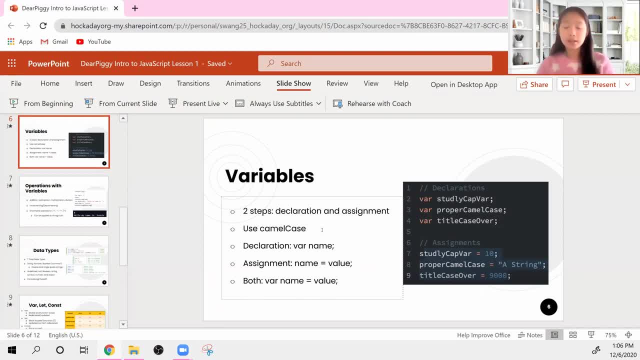 always a certain standard as to which everybody does their coding right, And then there's a standard for how you should name your variables. Camel case is where the first letter of the first word is lowercase, And then the other letters, the other words, their first letter is always. 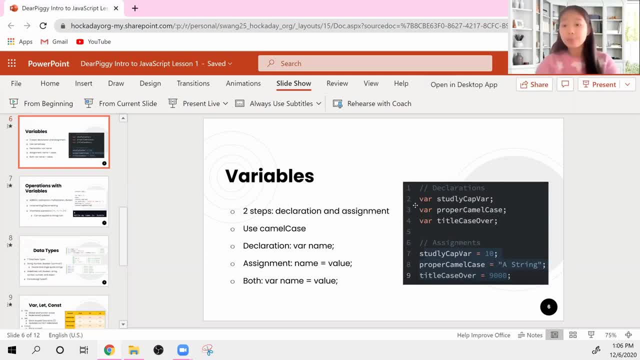 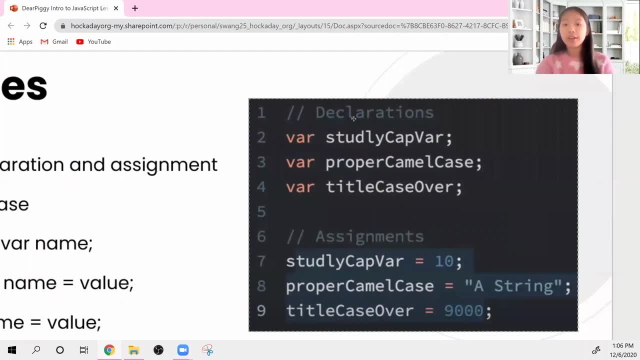 uppercase. So take a look at this picture over here. Not sure what these names are. They're very interesting names. Variable studly, cap var. proper camel case and title case over. You'll see that the first word of the variable is always lowercase. The first letter is always lowercase. 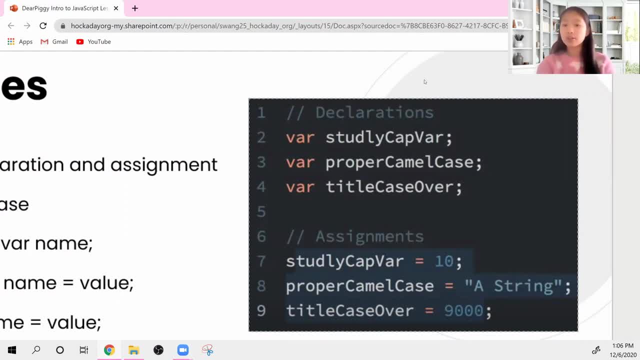 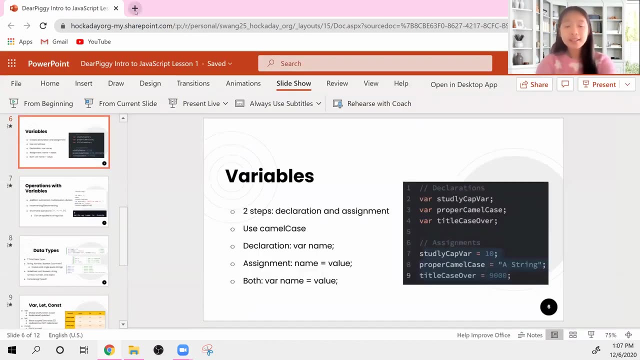 However, the second and third words, their first letter, is always uppercase. So first words, first letter, lowercase. all the other words, first letter is uppercase, And that's what we call camel case. Weird, right, I don't know why people use it, but we just have to go with it, right? So let's? 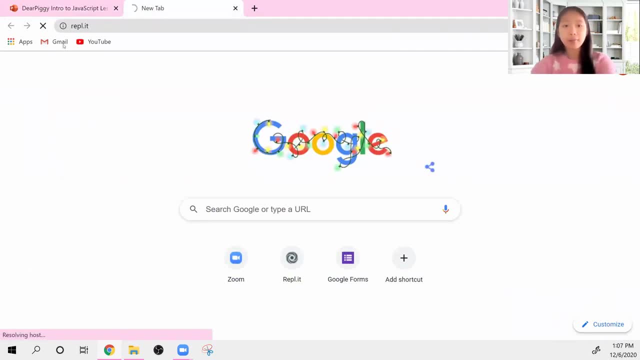 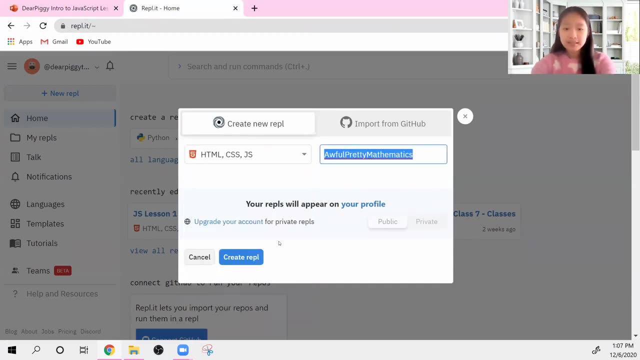 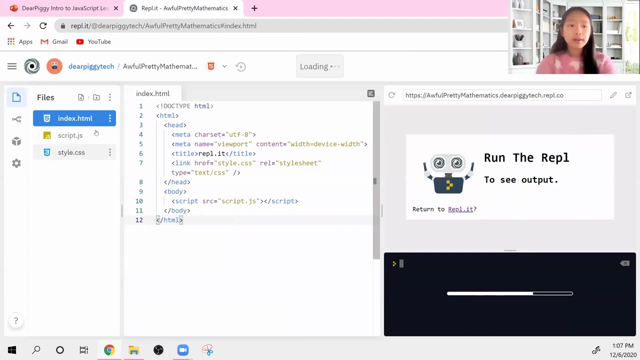 go ahead to REPLIT R-E-P-L-I, dot I-T, our in-browser, I-D-E, and we will create a new lesson, a new REPL, choose HTML CSS and create The REPL. So the first thing that we're going to do is we are going to go to our scriptjs and we 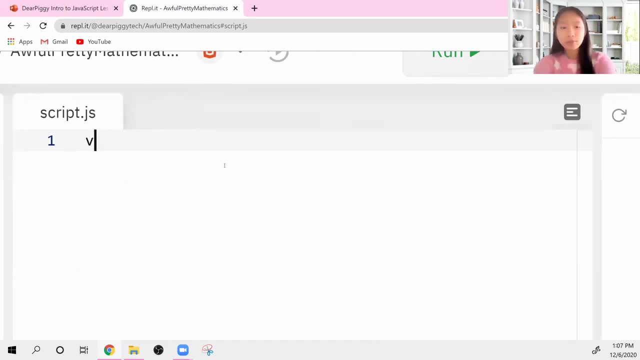 are going to create a variable And this variable var. we can say puppies var, puppies. it's equal to. let's see how many puppies do I want to have? I will have 17 puppies. Yes, I am a huge fan of. 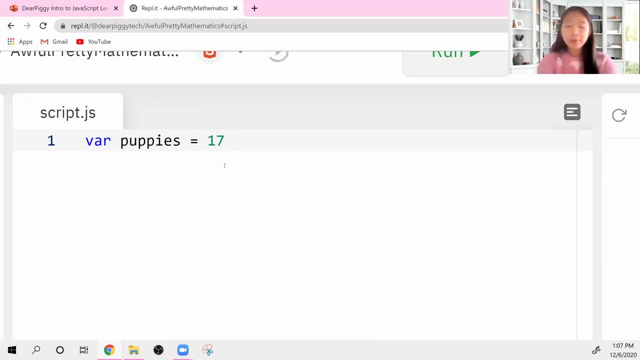 puppies. I really want a puppy, but I'm not going to have a puppy. I'm going to have a puppy, I'm not going to have one. But you know what? I think I would probably start with buying one puppy first, and then we'll build up to three, five maybe, then 17.. Might not try to get all 17 at once. 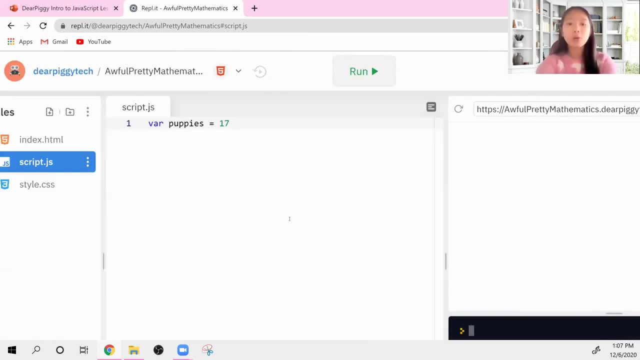 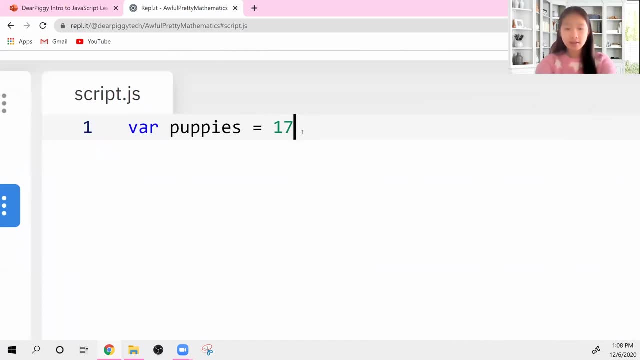 right. So now this is how we declare our variable in one line. Something that I want to note and point out to you is this ending over here. Right now, I have not added any sort of ending right, It's just 17, and then that's it. However, in JavaScript I have the option: 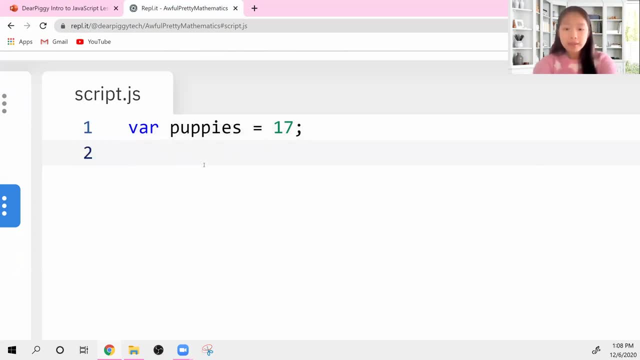 to add a semicolon at the end. So let me consolelog puppies And in this case, guys, we don't have quotation marks around the puppies because puppies is a variable. When you're printing out the value of a variable, you do not need to add quotation marks around it. 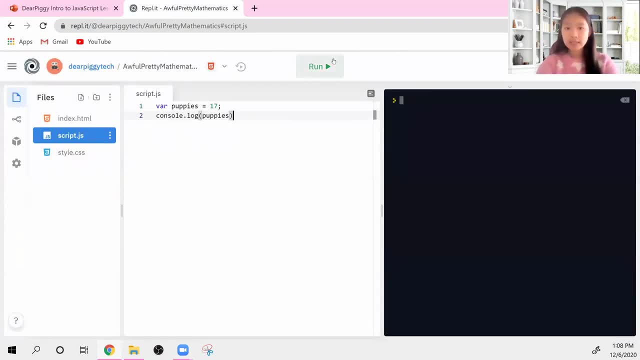 We run our code and in our console- let me drag this up- we see that it's 17.. So we see that this works fine. If I get rid of my semicolon here and then I run my code, we see that we still get. 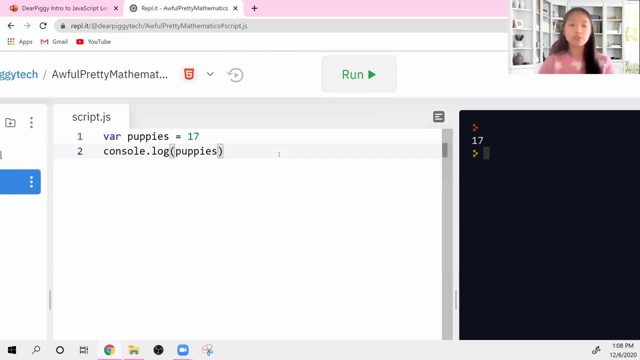 17.. So this is something that I really like about JavaScript Python, in my opinion, when they didn't, when they didn't have anything behind it, I thought that was a little bit too loose. Whereas Java, for example, a semicolon is required. you have to have it. I thought that was too strict. 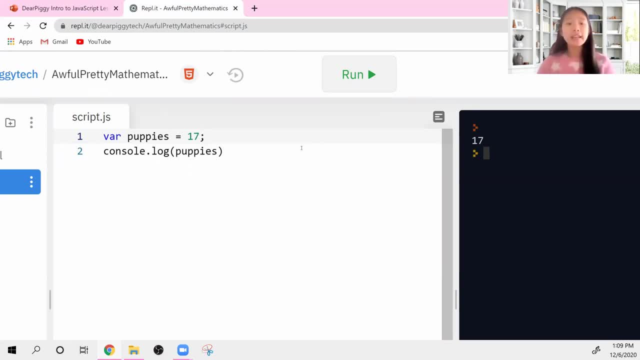 So maybe it's just me being picky, But personally I like how JavaScript allows you to put a semicolon if you would like. Now, I would always try my best to put a semicolon at the end of my code. So I'm going to go ahead and put a semicolon at the end of my code and then I'm going to. 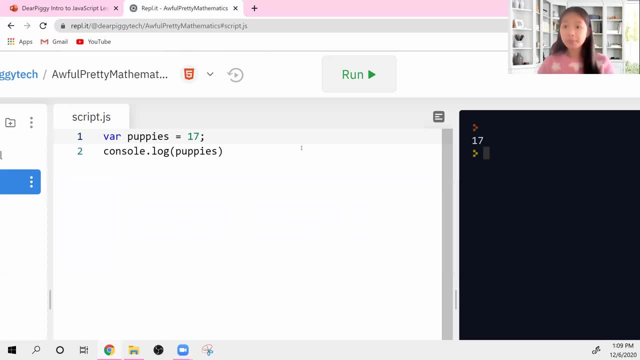 put a semicolon at the end Because in many languages, like Java and C sharp, these semicolons are required. So if you get into the habit of not putting a semicolon behind, then maybe when you move on to a different languages you're going to get an error message because you don't have a 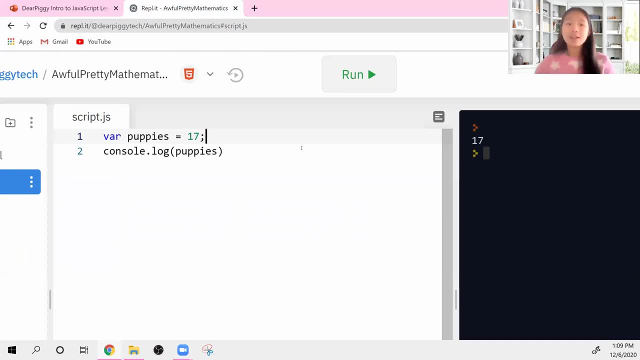 semicolon, So I would like to try to force myself to always put a semicolon at the end, just to get into a good habit of you know all coding languages, So we're going to use the semicolon at the end for now. Again, it's totally up to you though. 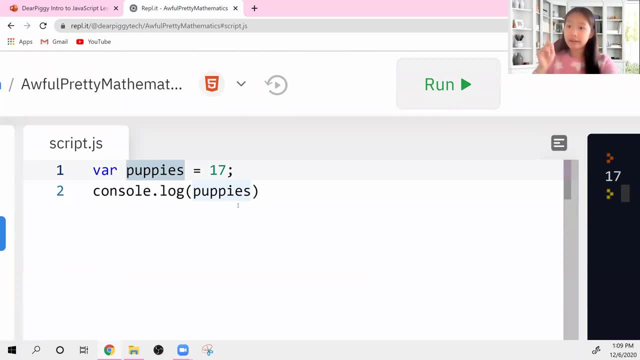 But my point is that we've just created our first variable and we've declared it and assigned it all on one line. Var puppies is equal to, with the value and the semicolon behind it. You could do it this way, or there's another way you can do it, Since we have to declare the variable and then 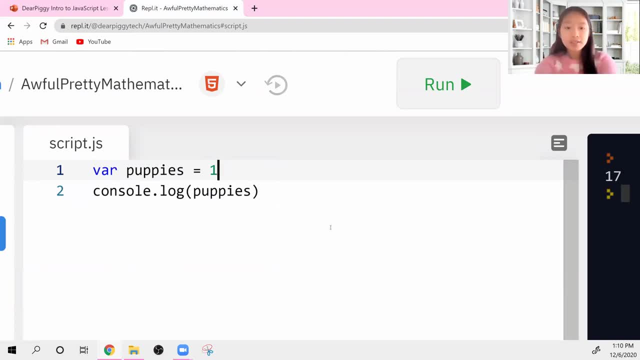 assign it. we can do this on two separate lines. So let's do this: Var puppies, and then you put a semicolon in the two separate lines here. Let's see, This will use comments declaration. This is where I declare that this variable exists, And the next line is where I assign it. where I assign a. 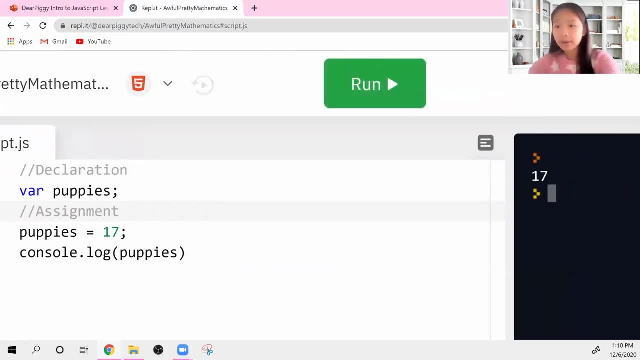 value to the variable And let's run our code and we see that we still get 17.. So everything is still working fine And I know some of you guys might be wondering why would you go through all the trouble of writing an extra line of code when everything could just fit on one line, That's. 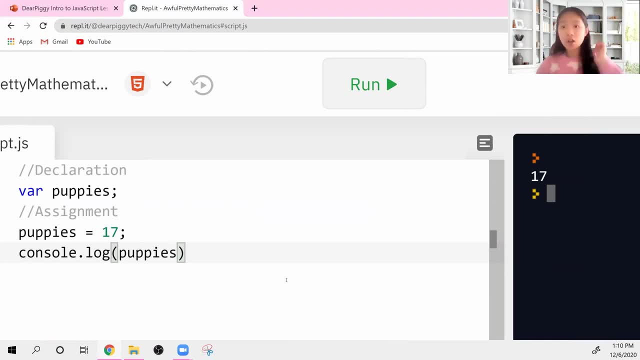 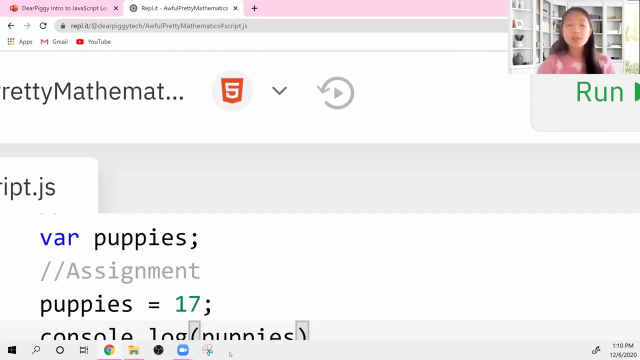 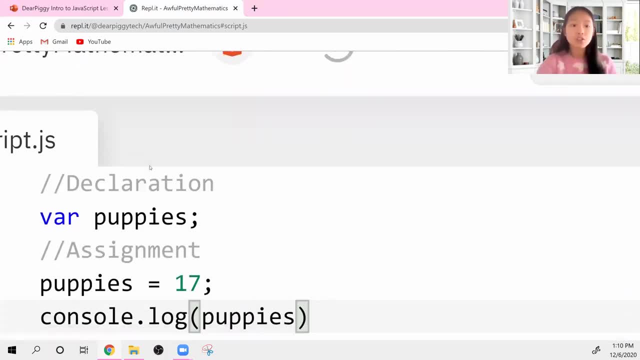 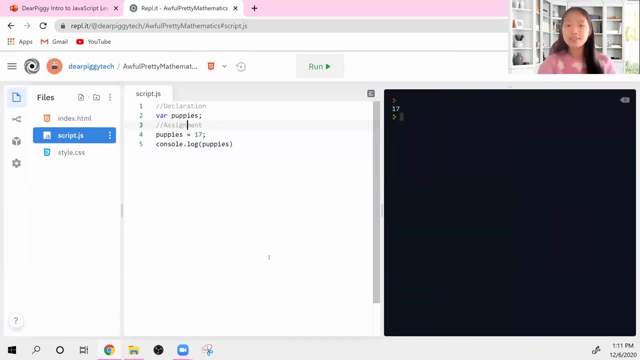 and more advanced. the value of puppies could change, So puppies will not always be 17.. So that is why you're allowed to declare it and assign it on two separate lines. We're always going to present all the options to you. you can feel free to choose whichever one you would like. 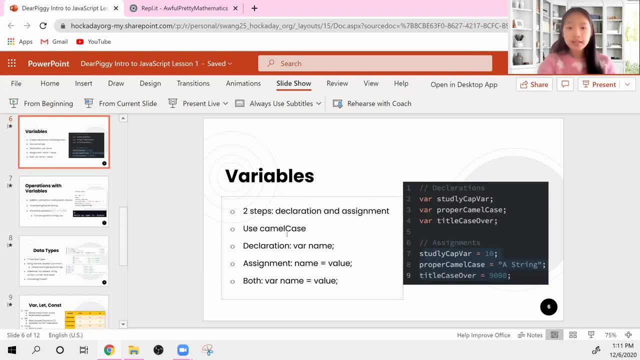 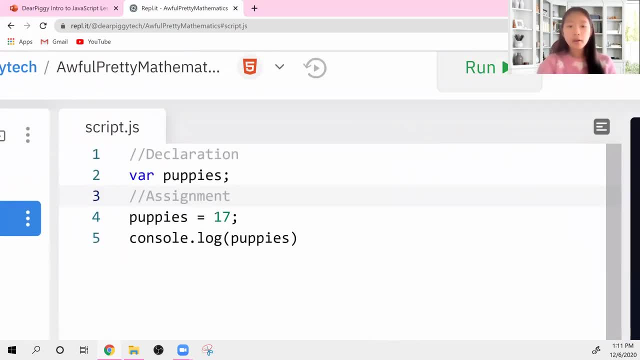 Let's see what else we need to talk about. For various reasons, we may want to know the main one. For example, we might want to know the number, your second name and your second name and not 2.. But that's not an option, So let's break it and 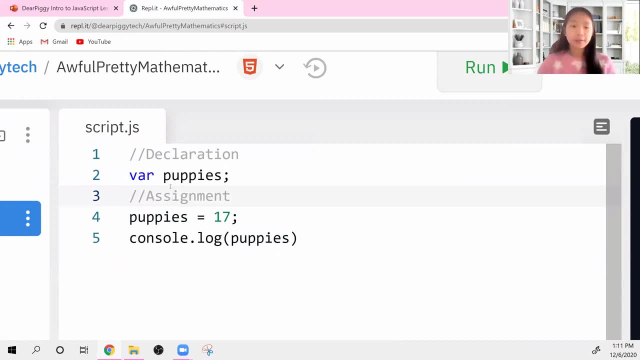 work it down. How many times can we say 1? 1,, 2,, 3,, 4,, 5,, 6,, 7,, 8,, 9,, 10,, 11,, 12,, 13,, 14,, 15,, 16,, 17,, 18,. 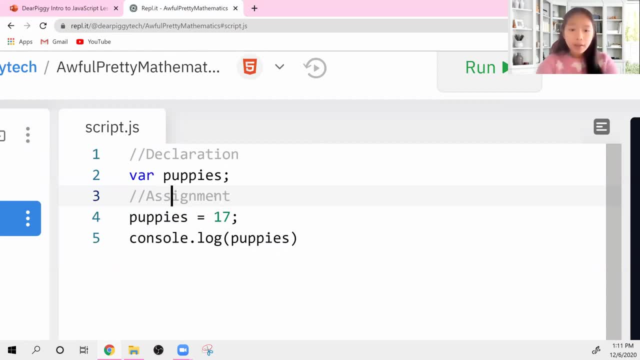 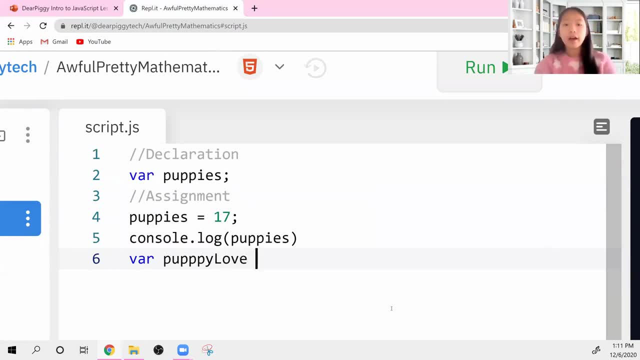 one word, it's just lowercase all the way through, right? In this case it's just one letter And so we've got the first one, which we call the lowercase, And those things that we can sit down and is camel case? right, because puppy is the first word. it's lowercase. the first letter is lowercase. 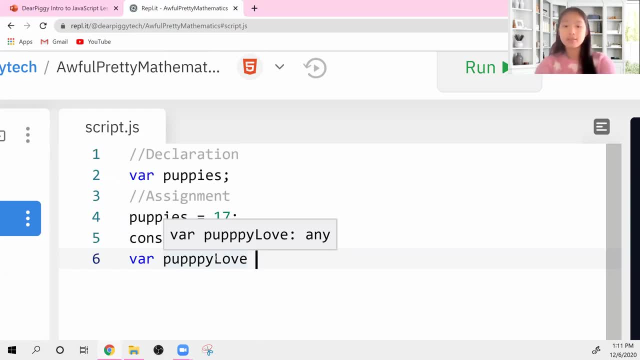 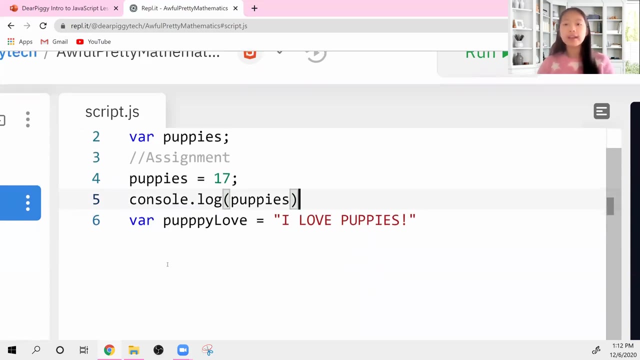 love is the second word, so the first letter is uppercase. so var puppy love is equal to i. i love puppies. okay, so this is where we kind of get a little bit of an introduction to data types coming in. now that is going to be. we're going to go deeper in just about like three minutes, but 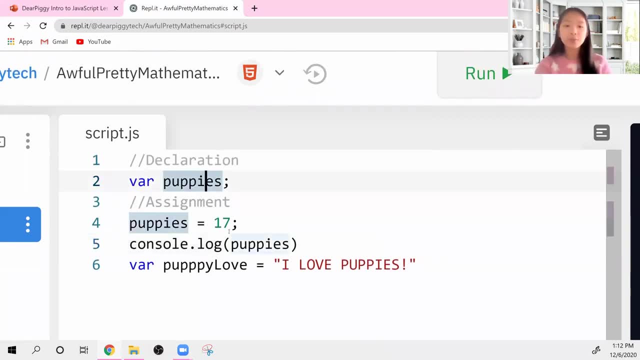 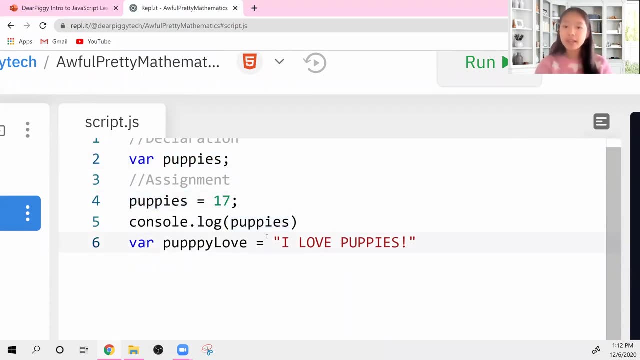 for now, i just want to show you that a variable can have whatever sort of value. in this case, puppies had a number as its value. in this case, we have letters. we have a string as its value. now, since it's a string, you need to put it in quotation marks. i had a great question. it said: 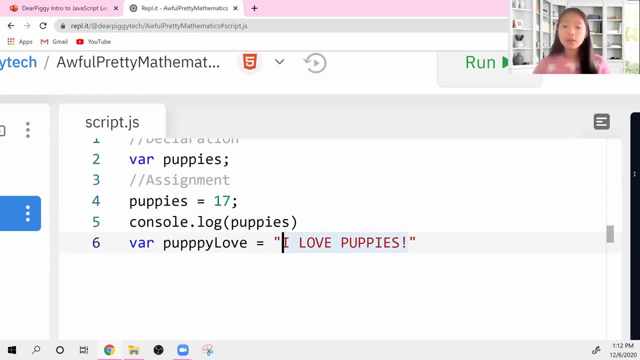 how do you know if something is a string? if you put quotation marks around it, then it is a string. if you don't, it's not a string. so these quotation marks, whether it's double quotes or single quotes, that is what makes some letters or some characters a string. so let's go ahead and 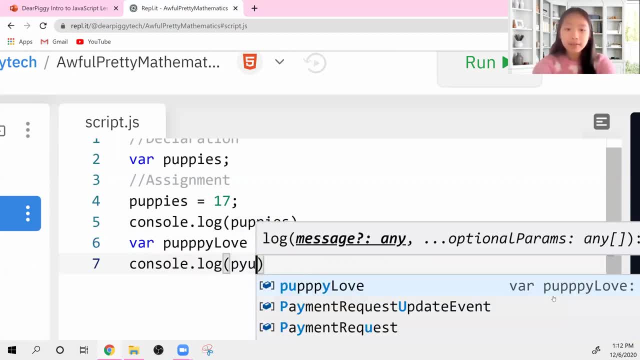 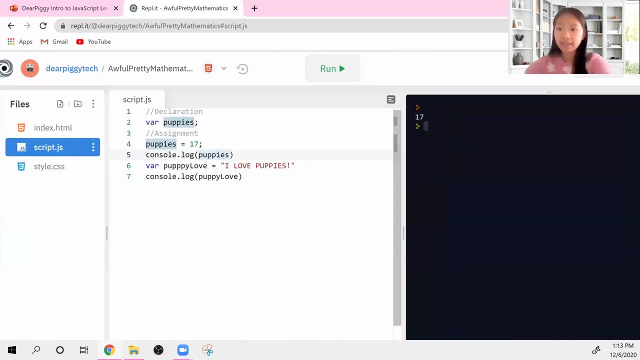 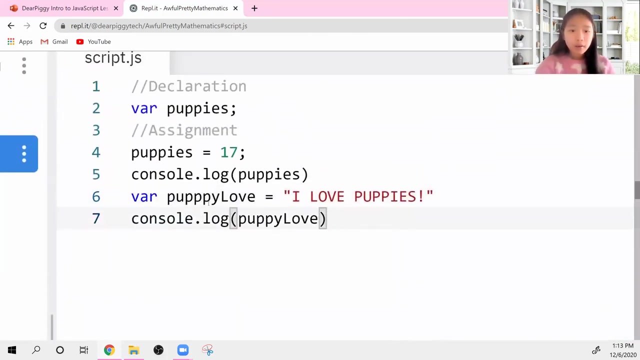 consolelog the value of puppy love, not puppies, puppy love, and we will run our code and let's see what happens. run and i have an error. puppy love is undefined, ah, okay. so guys, let's take a look here. what am i doing wrong? puppy love, ah, so this is not something. 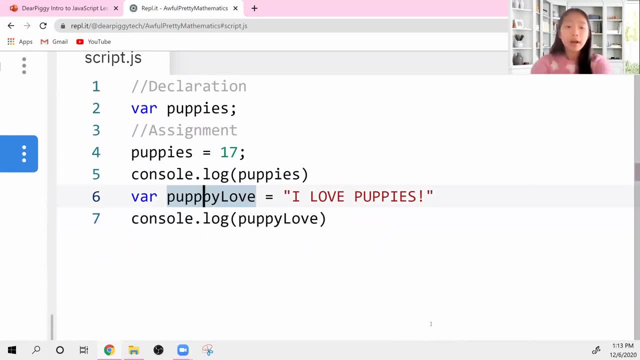 that i could have. most people can see very much, but, puppy, i spelled it wrong. i put three p's and i know i messed up. it's okay, but this is a great learning experience for everybody, right? your variable name is very picky- what you define it as when you declare your variable. 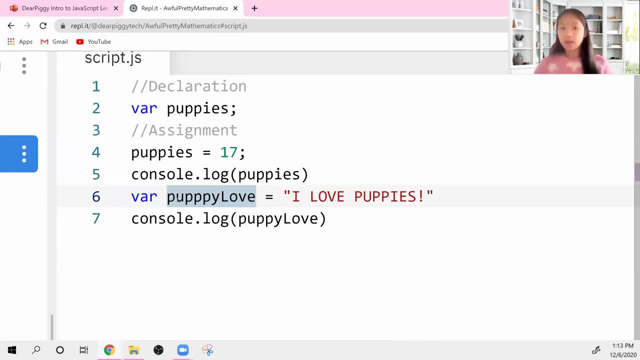 whether you spell it right or wrong. that is the name. you cannot put three p's over here and then two p's over here and expect it to work, because our program is not illiterate. it does not understand that you're trying to spell puppy, so now i'm going. 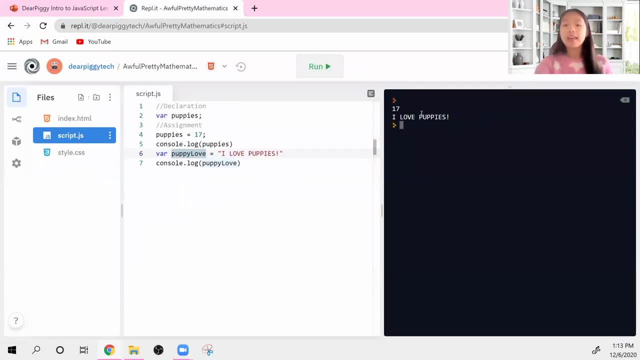 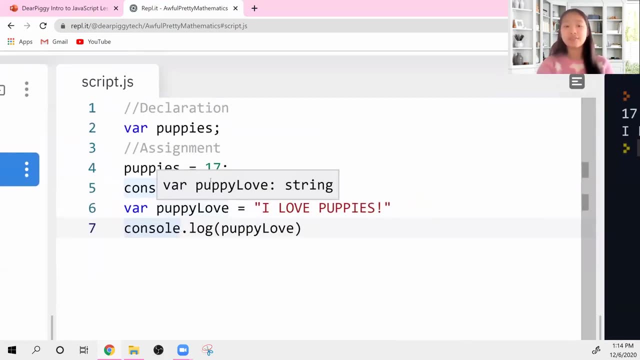 to make puppy spelled with only two p's and we run our code and we get the correct answer. i love puppies, so what? the mistake that i just made over? there was a great example of making sure that the variable name and the name that we use when we consolelog, when we print it to the console. 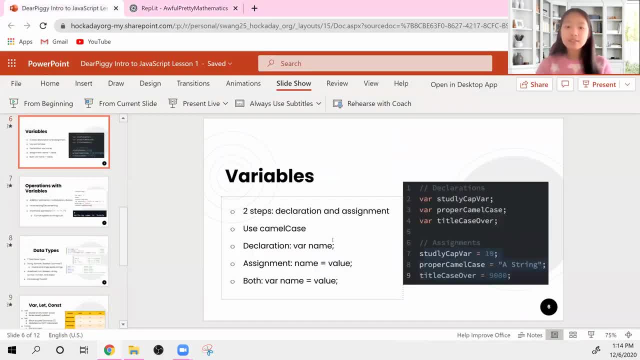 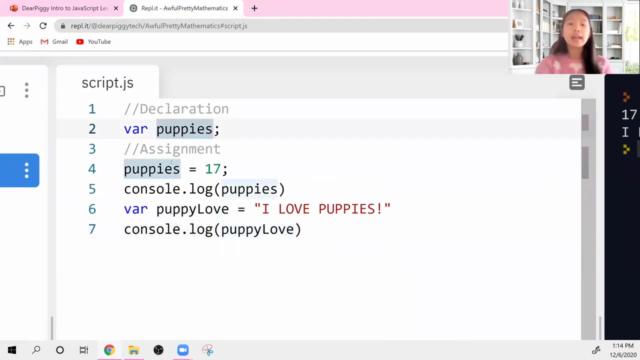 they both have to be the same. so that was variables in a nutshell. variables again. we used var the entire time and the reason why var is so good is because it can be redeclared and read and update it, which means that i can declare this again and i can update it however many times i want. that is one benefit of var. 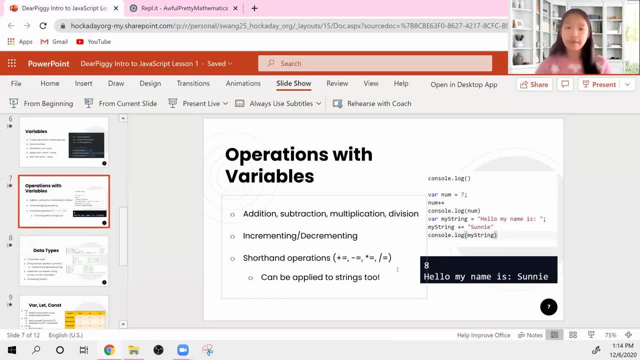 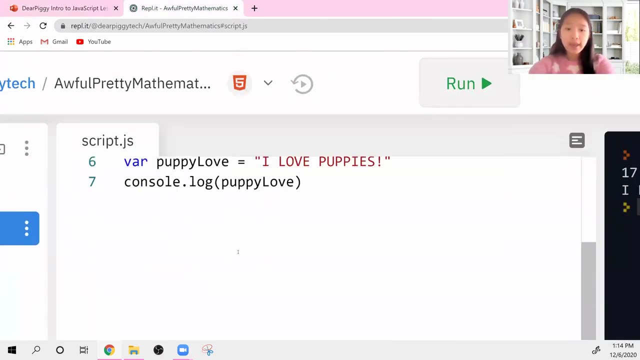 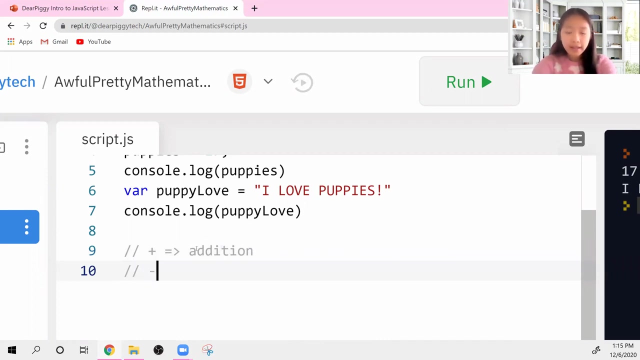 let's go on to operations with variables. now, just like math, we can do addition, subtraction, multiplication and divisibility with variables, assuming that these variables have a number value. and so let's just go ahead and use a comment. over here. we see that this plus sign stands for stands for addition, this minus sign stands for subtraction. 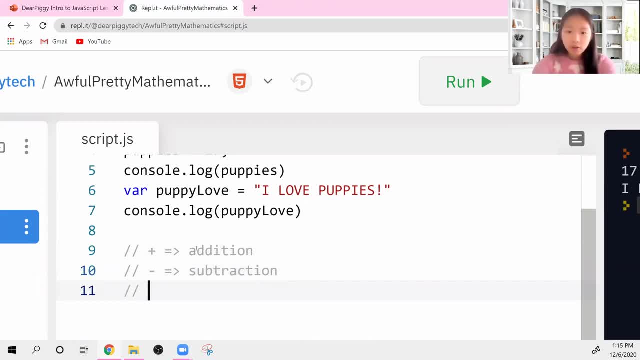 subtraction, which we all know, this asterisk, which is the top one on top of the eight, that stands for multiplication and this slash stands for division. another bonus one is mod division. it's the percent sign and that, essentially, is the remainder. now, if you guys don't know what mod is, that is totally okay, that's. 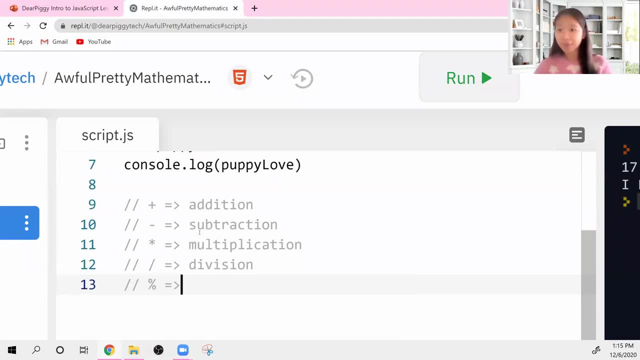 more of some thing that you understand as you guys learn about it in math. so once you guys learn about it, once you're old enough to learn about it in math, you will understand mod, but that means modulus, or which I like to just think of it as the 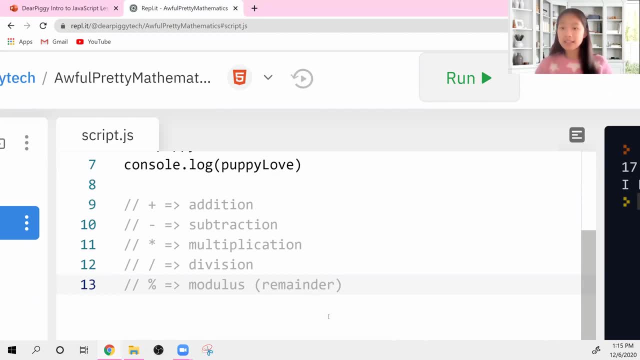 remainder. so this is kind of like our key. this is what these operations are. we don't need to review these because hopefully we've learned all of them. we were in pre-k. let's go over here and we're going to talk about incrementing and decrementing. 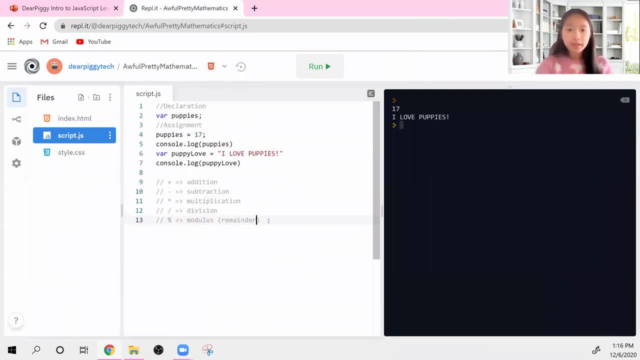 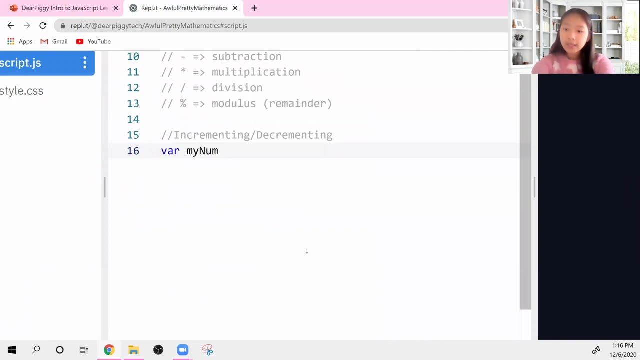 so I'm going to come over here and I'm going to create- I'm going to say we're going to work on incrementing slash decrement. now I'm going to create my own variable again and I'm going to sign it into- clear it in one line: VAR myno again. 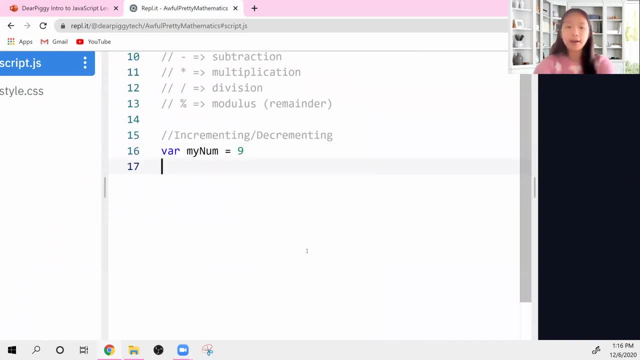 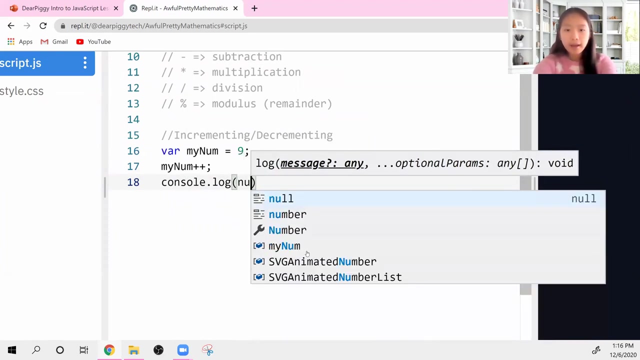 using camelcase is equal to: let's just use nine now. now, guys, what do you think would happen if I did mynum++? So some of the kids, and let me print out the value to the console: console, the log, my, my mynum. 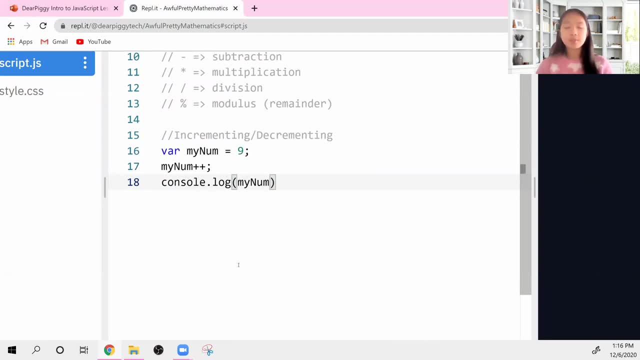 Okay, there we go. So some people said plus plus would give you 81.. Some people said plus plus would give you 27.. And I all understand where those are coming from. right, It makes complete sense. Some people think you're doing it to the power. 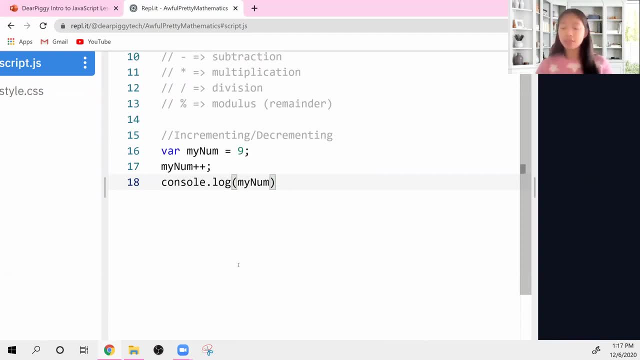 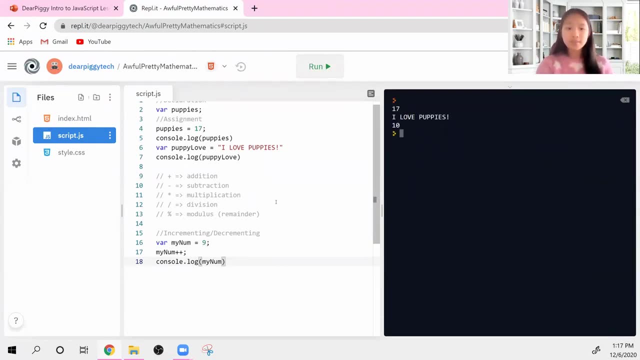 Some people think you're multiplying. Some people said 11.. They thought you were adding 2.. It's actually kind of weird guys. It's going to give you 10.. And the reason why is because if you do plus plus, it basically says add 1.. 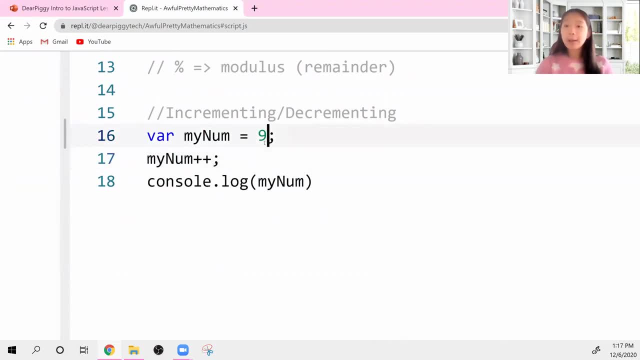 So whatever variable, plus plus would be the value plus 1.. So that's just something to remember Now over here. mynum, minus, minus, And then let's consolelog. So mynum again. most of you guys, some people actually did think that we were going to get 9.. 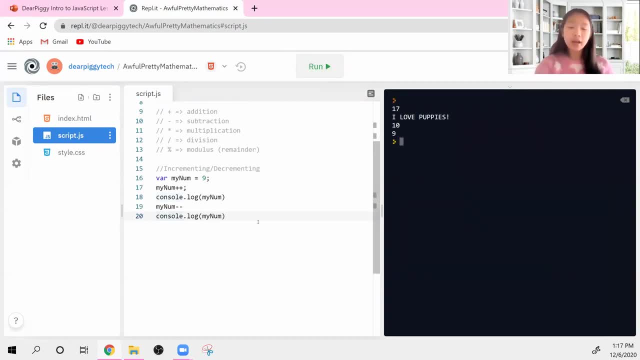 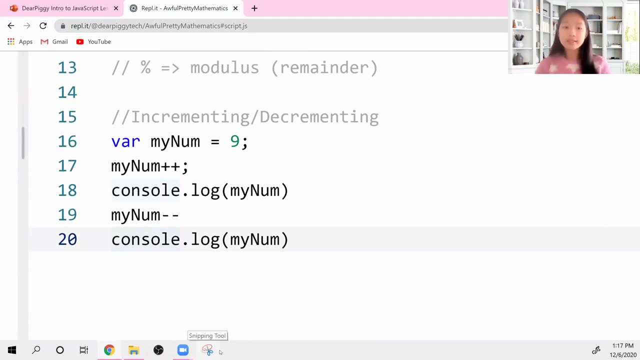 Some people, we're going to get 9.. Yes, that's the right answer, But some of you guys thought that we would get 8.. Now, this is where we really want to go over the order in which the program looks at our code. 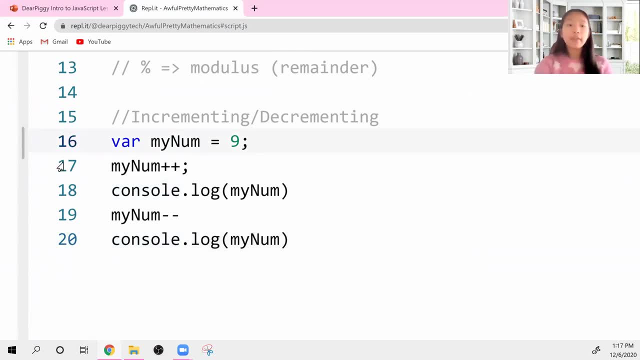 On line 16, mynum is equal to 9.. On line 17,, since we added 1, mynum is equal to 10.. On line 18, mynum is still equal to 10. Except we just printed 10 to the console. 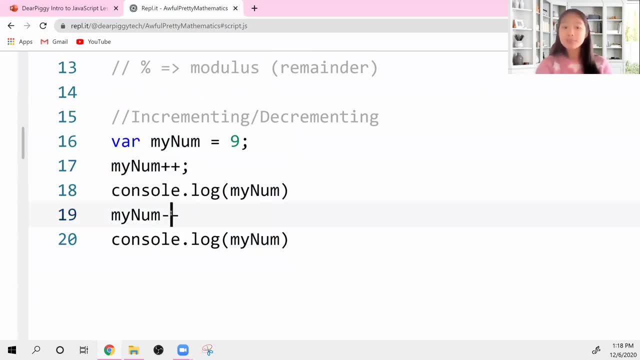 Since we know that plus plus is plus 1, we're assuming that minus minus is minus 1, right, But since at line 18, mynum had a value of 10, when you subtract 1 from 10, mynum is now back to 9.. 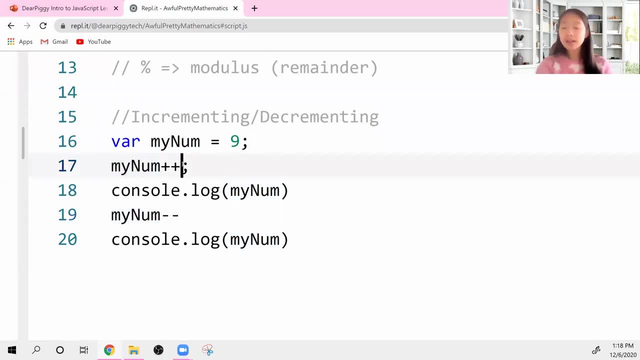 So this mynum minus minus and mynum plus plus balances everything out. So by looking through this line by line we kind of see that it goes in chronological order. So that was incrementing and decrementing. Pretty easy to understand, I would believe.